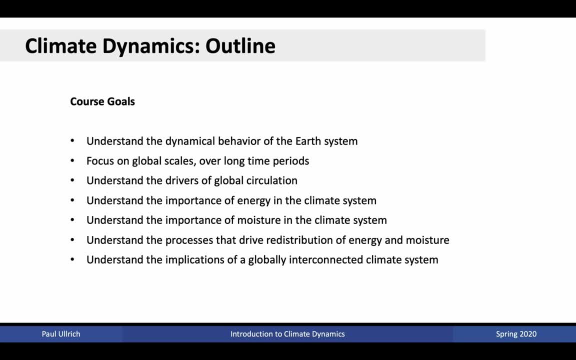 the large-scale behavior of the system and, consequently, the fine-scale weather features that we see in our everyday lives. Finally, we're going to understand the implications that come about as a consequence of this globally interconnected climate system and how, for instance through our own behavior, we're able to influence the global climate system. 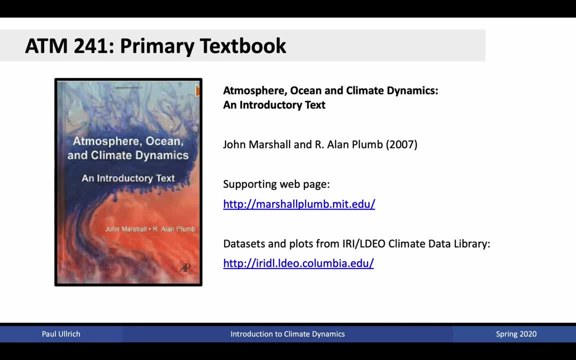 The textbook for this class is Atmosphere, Ocean and Climate Dynamics, an Introductory Text by Marshall and Plum. The supporting webpage can be found here As well. datasets and plots are available from the Columbia IRI-LDEO Climate Data Library, available here. 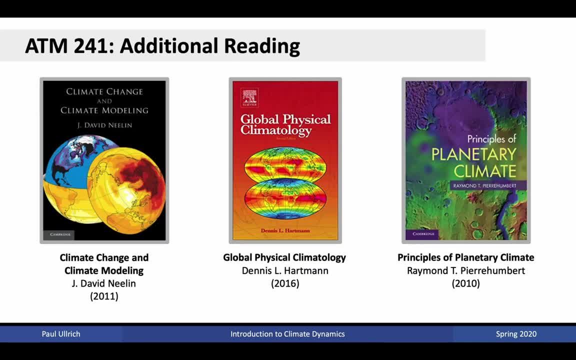 Additional reading that could supplement your learning through this course include Climate Change and Climate Modeling by David Nealon, Global Physical Climatology by Dennis Hartman, and Principles of Climate Change and Climate Modeling by David Nealon. All of these books are excellent reference material and are highly recommended if you 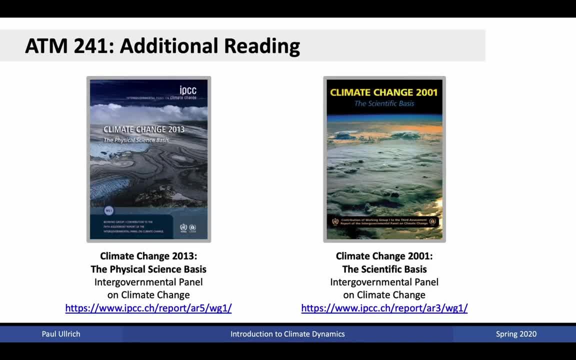 want to expand on your knowledge of climate dynamics. In addition, I highly suggest turning to the IPCC Assessment Reports for an understanding of the global climate system. These two assessment reports, in particular- AR5 here on the left and AR3 on the right- both have extensive chapters. dedicated to the global climate system. These two assessment reports in particular- AR5 here on the left and AR3 on the right- both have extensive chapters dedicated to the global climate system. Remember to see them at the beginning of the show, just to review what is correct and what is wrong. 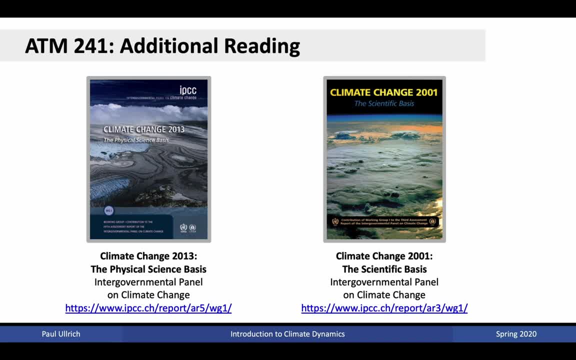 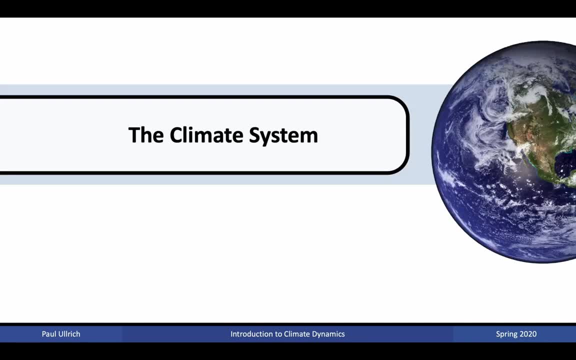 In particular, if you are interested in learning more about the global climate system, I do recommend the second assessment of the global climate system, as well as the third assessment for further learning. All right, let's dive right into understanding the global climate system. 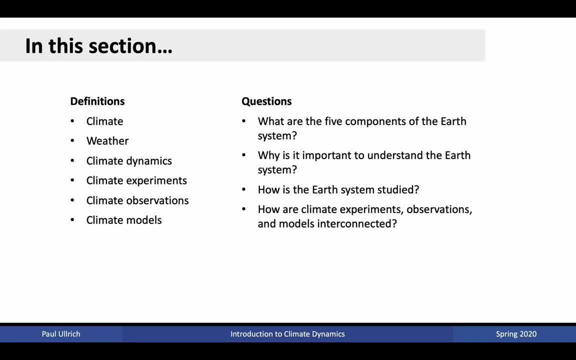 In this section, we're going to learn definitions of climate weather, climate dynamics, climate experiments, observations and models. We're going to answer questions that include: what are the five components of the Earth system, why are they changing, how do we interpret them, what are they affecting us and why is climate紀メ? Authorities would like American Climate risque only to include reality. 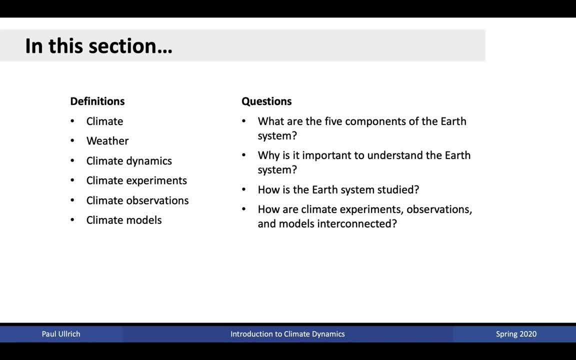 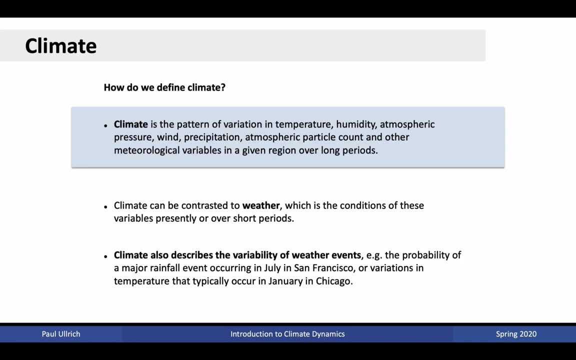 Why is it important to understand the Earth system? How is the Earth system studied, And how are climate experiments, observations and models interconnected? So before we proceed, we need to define what exactly climate is before we can understand its dynamics. The common definition of climate is that it's the pattern of variation in temperature, humidity. 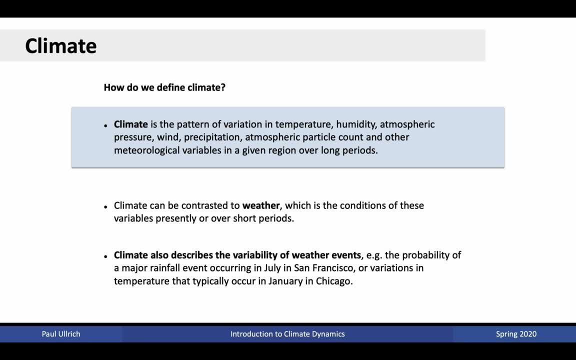 atmospheric pressure, wind, precipitation, atmospheric particle count and other meteorological variables in a given region over long periods. Here meteorological variables refer to characteristics of the atmosphere and point-wise one can say these are associated with characteristics of individual weather events. 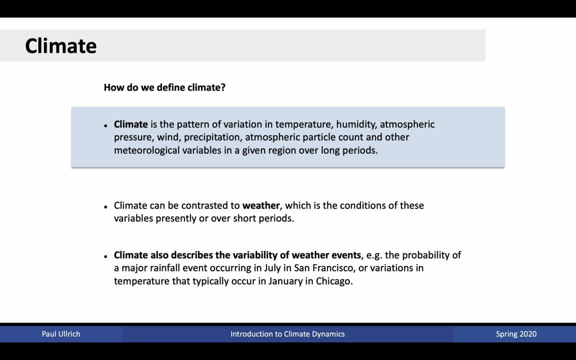 So we're going to take individual weather events and basically average them over very long periods in order to understand their statistics. This is in contrast with individual weather events, which are, of course, point-wise samples. This is effectively similar to climate describing a large-scale statistical. 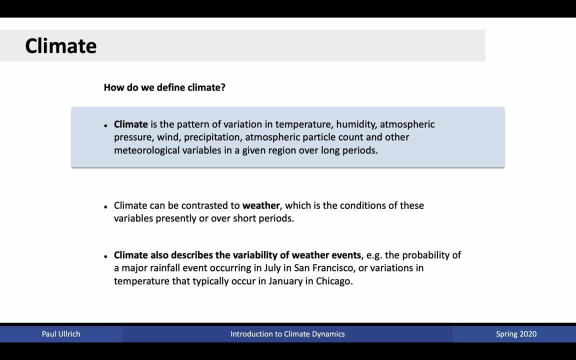 distribution of weather, whereas weather is simply one sample taken from that distribution at a given time. Weather, in particular, are the conditions of meteorological variables that are at a single point in time, such as presently, or that occur over short time periods. Notably climate also describes the variability of weather events. 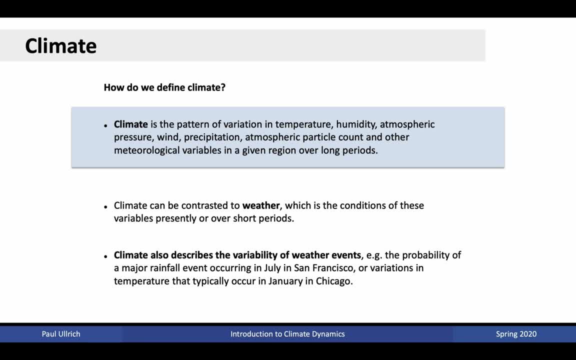 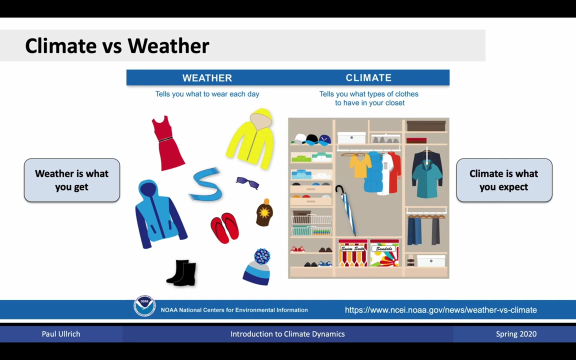 So, besides simply describing the average weather, one can also investigate the distribution of weather. For example, what's the typical range of temperatures that might occur in San Francisco, What is the probability of a major rainfall event occurring, Or what types of weather systems are generally found at a particular time of year? 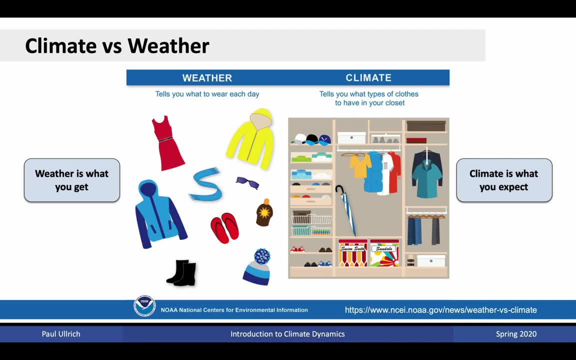 The typical NOAA dichotomy when it comes to weather and climate is: weather is what you get and climate is what you expect. If you look at your closet, the types of clothes that you have in your closet are likely to be more or less similar to what you get in your closet. 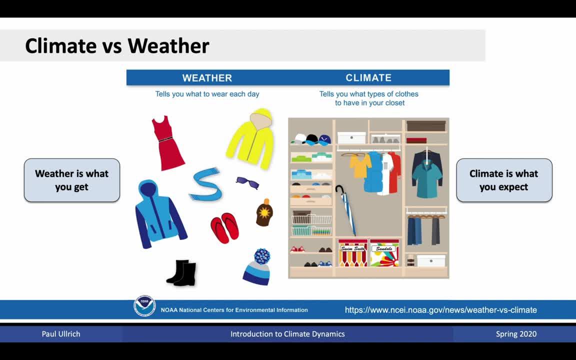 You can also look at the number of clothes that you have in your closet, and the number closet for going out around your house on an everyday basis describes the climate of your region. If you live in a warm region, you'll typically have short-sleeved shirts, maybe. 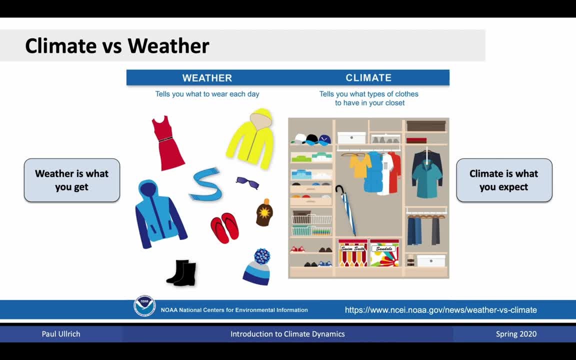 swimwear, whereas if you live in a cold region, you're going to typically have heavy jackets, long-sleeved shirts, sweaters, etc. So, while you expect particular weather events to occur, you will then have the clothes available in order to be prepared for those individual weather. 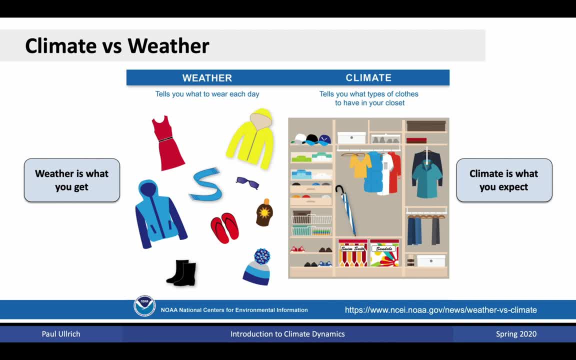 events. The clothes that you wear every day or on a particular day are then descriptive of the underlying weather. If it's raining out, you typically wear a rain jacket. If it's warm out, you typically wear a short-sleeved shirt. These are, of course, drawn from the climate or drawn 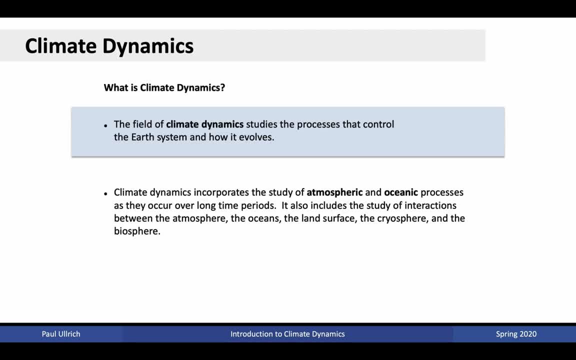 from your closet, which is the descriptor of the climate. So what is climate dynamics then? The field of climate dynamics specifically studies the processes that control the earth system and how it evolves. That is, we're investigating the large-scale statistics of the earth system, and so we want to investigate. 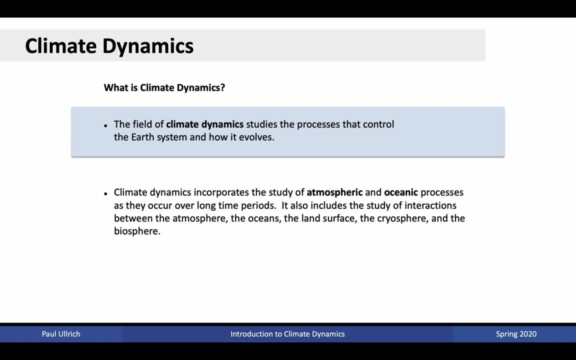 the processes that give rise to these particular statistical distributions. This incorporates the study of both atmospheric and oceanic processes, as well as the interactions between these components of the climate system. As well, they investigate interactions that occur between the atmosphere and land surface, the cryosphere and the biosphere, So there's many different components. 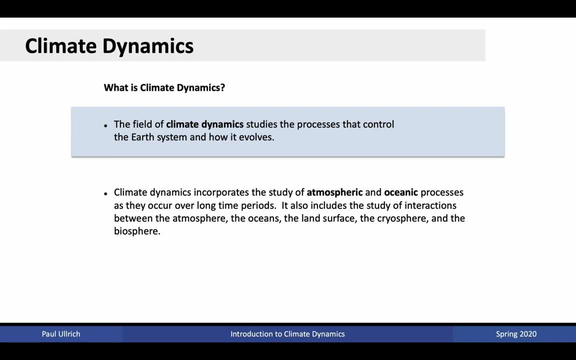 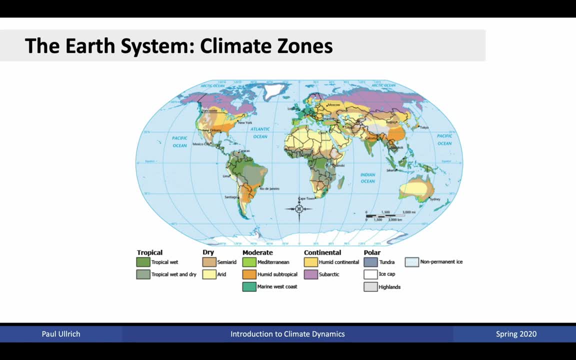 present within the earth system that are investigated. Let's look at climate zones that cover the planet. You may be familiar with this from staring at a map, but it's kind of common knowledge that if you go towards the equator you're going to find typically warmer temperatures, and as you go towards the 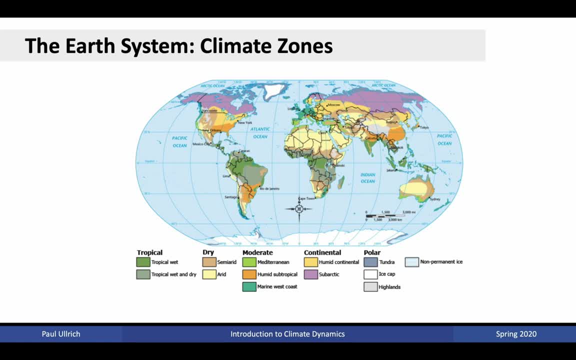 poles, you're going to have cooler temperatures. Also, we know that the deserts of the world are typically located around 20 degrees north and south, and that the mid-latitudes have kind of their own distinct weather regimes. So what we can do, then, is delineate different climate zones across the world based on typical. 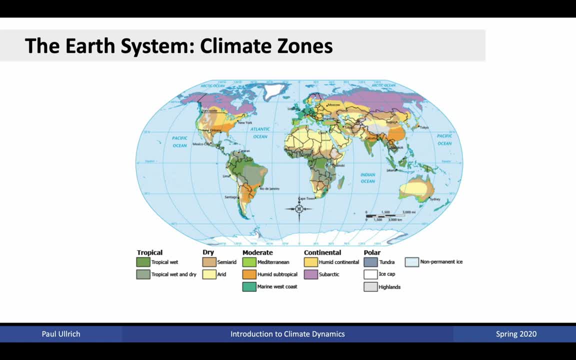 temperatures and precipitation. So if you look in the tropics along the equator, you expect to find tropical climates. If you go to the subtropics, such as at 20 degrees north, you expect to find arid, desert-type climates. 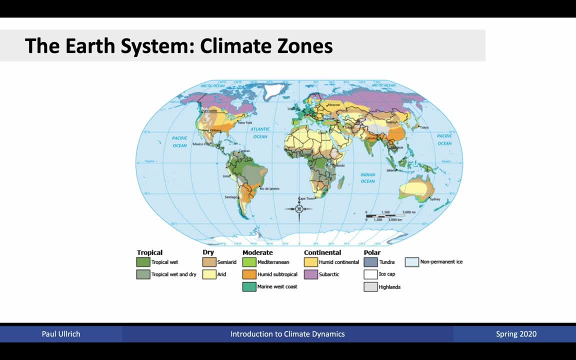 In the mid-latitudes you can have Mediterranean climates, humid, subtropical or marine, west coast-type climates, And if you go farther inland you might find continental climates as well. The distribution of land, the distribution of water. how far you are from the equator? 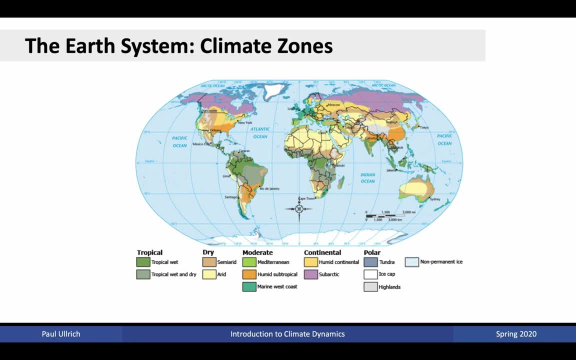 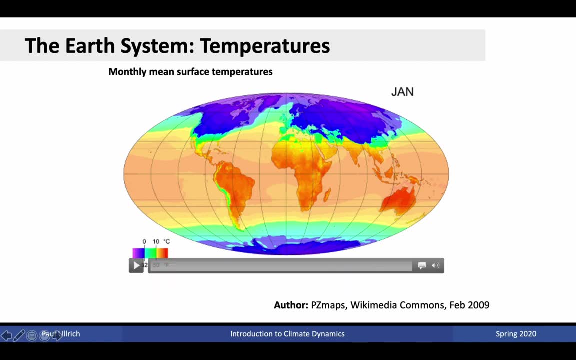 all play a role in determining the underlying climate that you experience. Let's look at the temperature variations of the earth system. In Manewari, we typically find that temperatures are warmer south of the equator. This is because the sun is, of course, located south of the equator at this time and 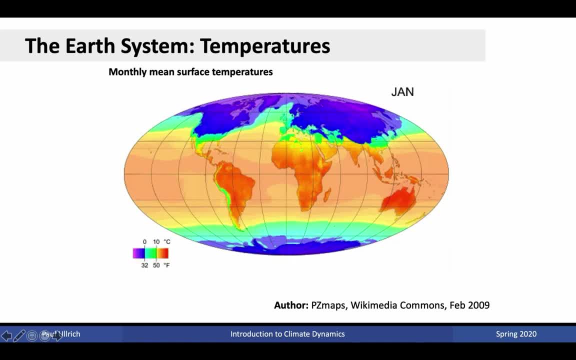 summer. As the sun progresses through this oscillation throughout the year, we have a slow tendency towards warmer conditions in the northern hemisphere- summer in the northern hemisphere- and corresponding cooler conditions at the same time. Similarly, during the southern hemisphere, summer, we find warmer conditions in the south and cooler conditions in the north. 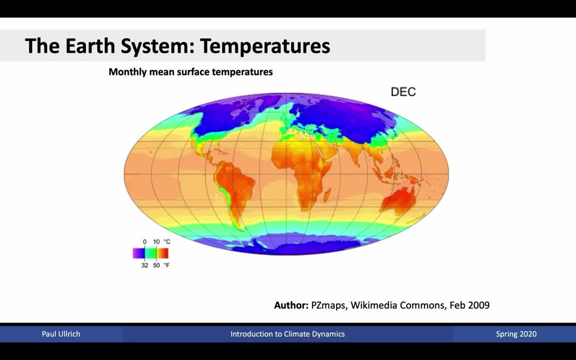 Other observations that we can make from examining this plot is that temperatures tend to be cooler over land and further, what we see is that the variation in temperature appears to be far more modest over the oceans. This is one of the reasons, for instance, why California experiences. 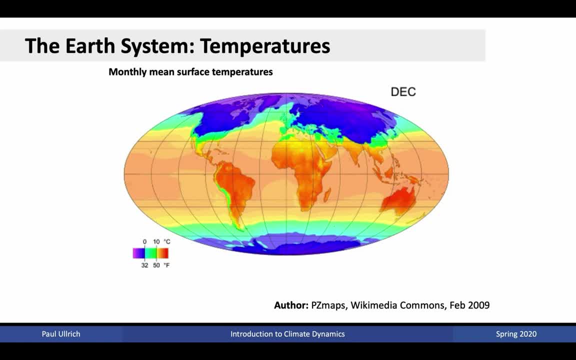 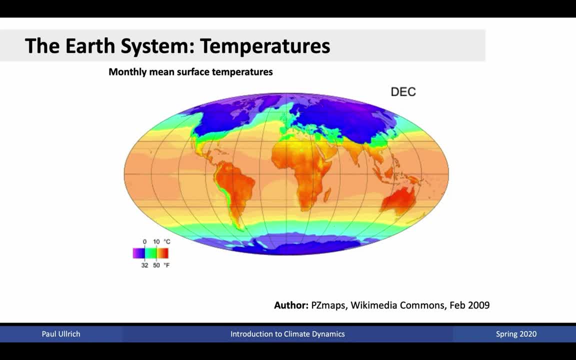 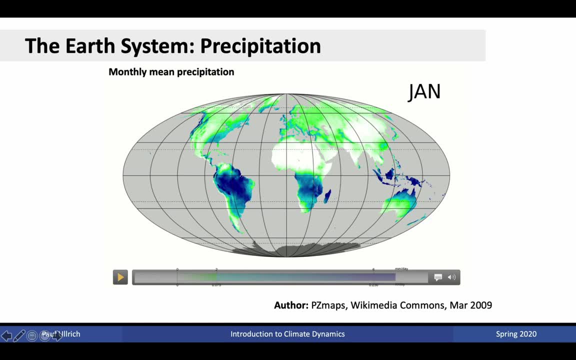 system is that, of course, you have temperatures that tend to decrease from equator to pole. Let's now turn our attention towards precipitation. Precipitation has a slightly different character associated with it. It's no longer clear that there's a single variation. 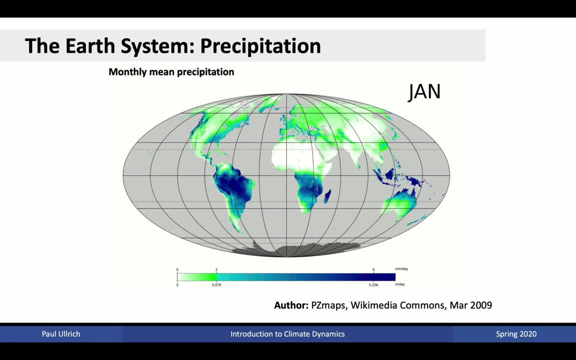 for instance, from equator to pole. Instead, what we see in a typical January is that precipitation tends to be very heavy in equatorial regions, in the tropics, in the rainforests of the world, and it's also very heavy, for instance, along the west coast of. 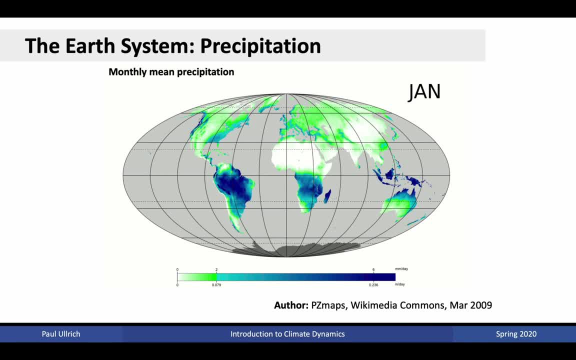 the continents and, to a lesser degree, in the southeast of the United States. As we progress through the year, however, we do see some shift in this underlying pattern. If you pay close attention to the behavior of precipitation in the equatorial regions, what you will see is: 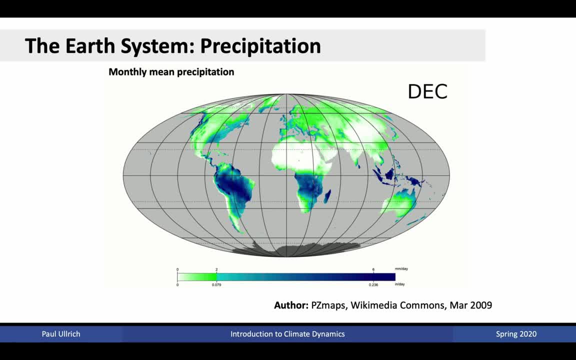 that there appears to be a northern shift through the summer season that then moves back south into the north through the northern hemisphere winter. This pattern of precipitation through the equator then does follow the pattern of temperature that we've seen in the previous plot. However, there are other characteristics associated with precipitation here as well. 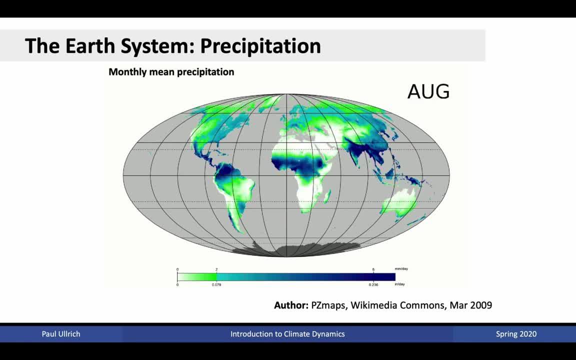 If you stare at the west coast of the US, what you will see is that through the summer season you obtain drying that has moved northwards from the arid regions of the subtropics, whereas in the winter season the wetter northern regions have moved southwards. 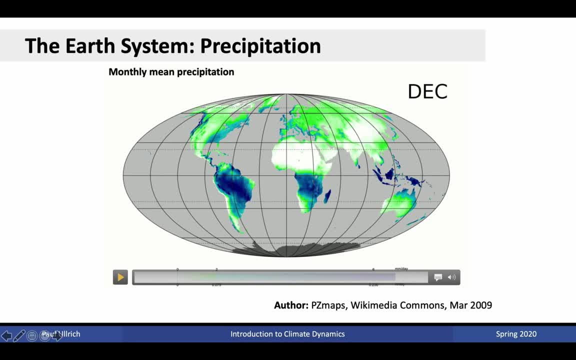 Further. if you look at, for instance, the southeast Asia or in the Indian region, what you will see is that there is significant precipitation associated with the migration of the monsoonal systems. These regions, of course, experience heavy precipitation at certain times of the year associated with the monsoonal migration. 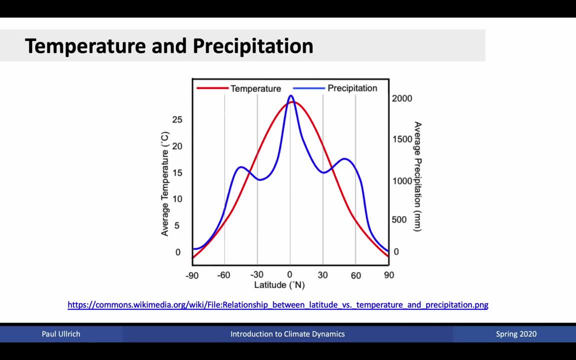 If we were to plot the annual temperature and precipitation rate of the year, we would see that if we were to plot the annual temperature and precipitation on top of one another, what you would find is that the temperature is essentially a unimodal distribution. 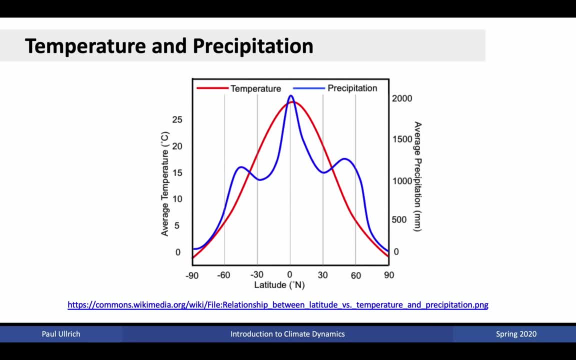 It's peaked around the equator and it is minimum at the poles. Precipitation, on the other hand, has an interesting trimodal distribution. So, whereas precipitation is maximal around the equator, it also has two peaks in the mid-latitudes, as well as dry regions in between. 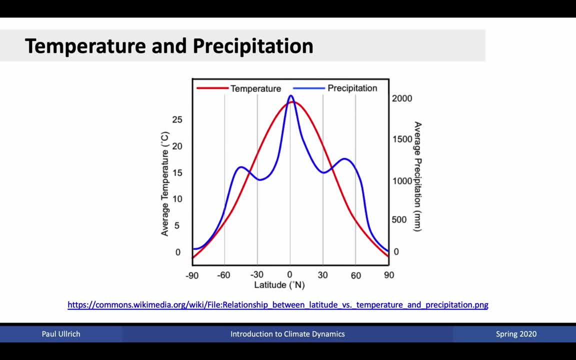 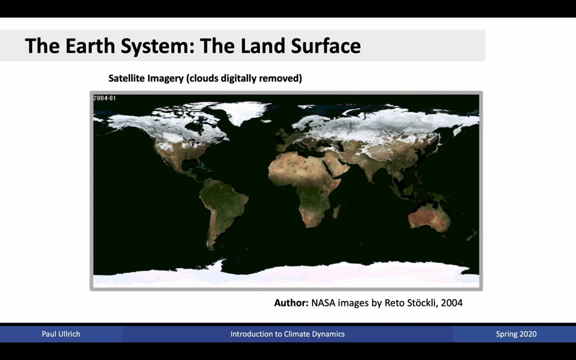 The driest regions of the world, where precipitation is minimal, also occur in the mid-latitudes. So in the mid-latitudes there is a lot of precipitation that occurs at the poles. Let's look at the land surface. Here on this plot, we can see a satellite image with clouds digitally. 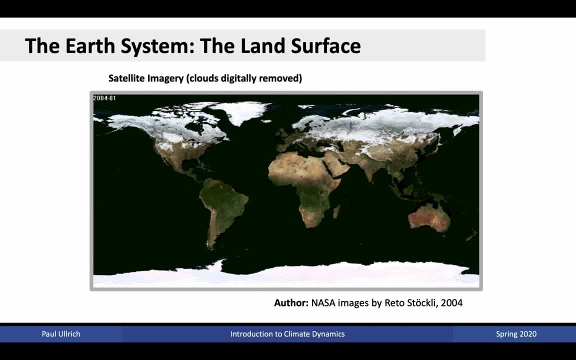 removed, We see colors representative of vegetation, dryness and snow all over the earth. What I want you to pay attention to in this is the behavior of vegetation and snow as we progress through the season. In particular, what you'll notice is that as warmer conditions move up through the northern, 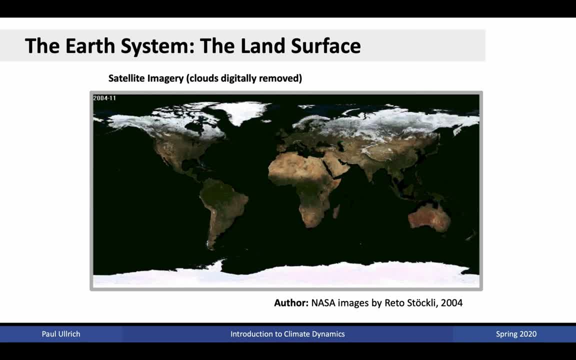 hemisphere. through the summer season, snow recedes farther to the north. This is because the warmer conditions melt the snow as we move into the summer season. However, in other places of the world, we also see variations that are seasonal. Pay attention to the behavior of, for instance, 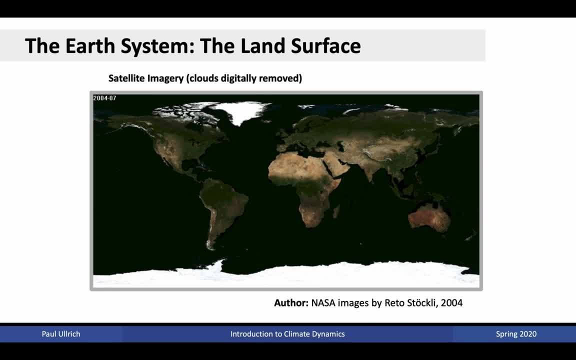 the rainforests of Brazil or the green regions of central Africa. What you'll notice is that as we move through the summer season, these regions see some change in. arguably, the regular weather tend to follow along with the point of maximum precipitation and temperature, That is we see. 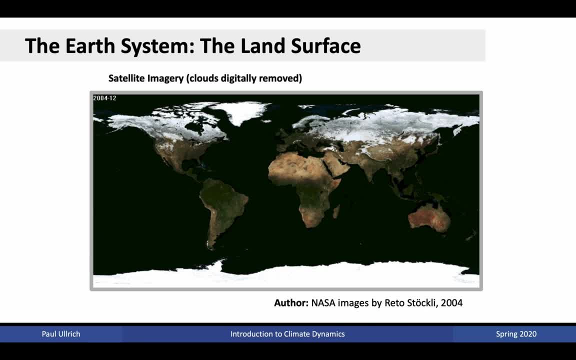 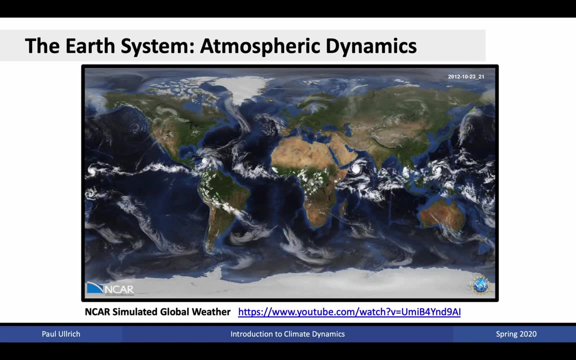 greening move farther north through the northern hemisphere, summer, and drying occupy those regions as we enter into the northern hemisphere, winter. The dynamics of the atmosphere explain individual weather systems, and these dynamics are in response to the large-scale drivers of the climate. The temperature that we observed previously is primarily driven by the behavior of the sun, as 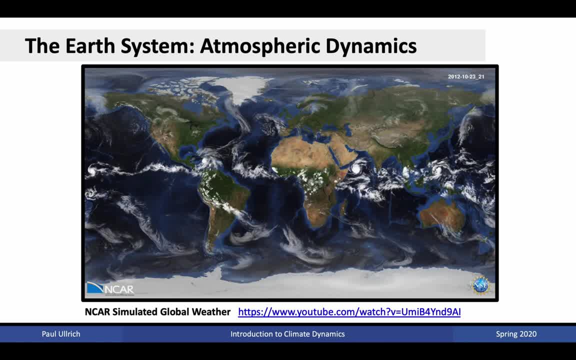 it moves through the year. Precipitation responds in part to that warming from the sun and as we evaporate water vapor into the atmosphere, we get the formation of clouds and we drive the dynamics of the global atmosphere. If you want to see a simulated Earth's atmosphere, I will refer. 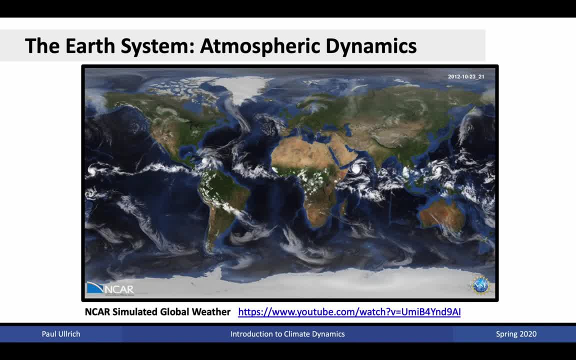 you to the YouTube link shown here. It shows a high-resolution video where individual weather systems and cloud patterns are resolved. Some of the key features you will be looking for include the tropical band, where you'll notice large convective plumes associated with point-wise clouds. You'll notice large whip-like objects in 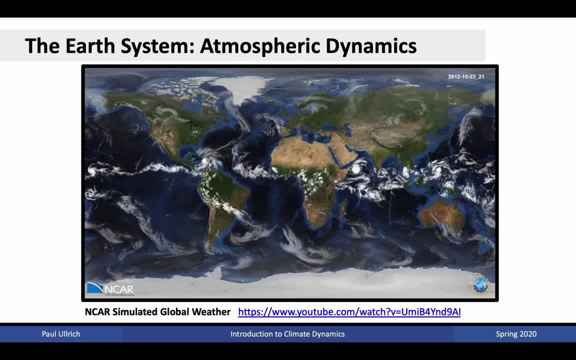 the mid-latitudes, known as atmospheric rivers, where clouds and moisture are transported poleward and are responsible for giving rise to the large precipitation that occurs along the western edge of continents As well. you'll notice things like tropical cyclones and other atmospheric 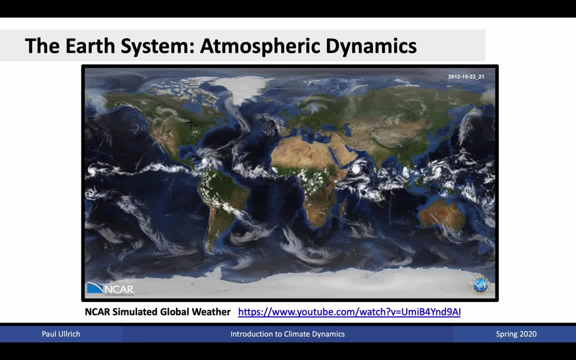 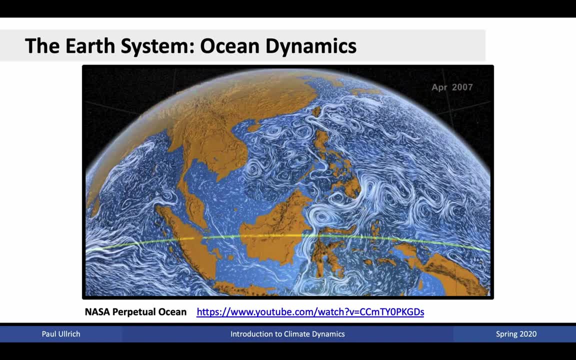 features that are responsible for driving day-to-day weather. If you look at the ocean, the ocean itself is a dynamic beast as well. The NASA perpetual ocean provides an excellent view into the movements that occur within the ocean. The ocean is driven by large-scale circulations, known as the oceanic gyres, as well as small-scale eddies that 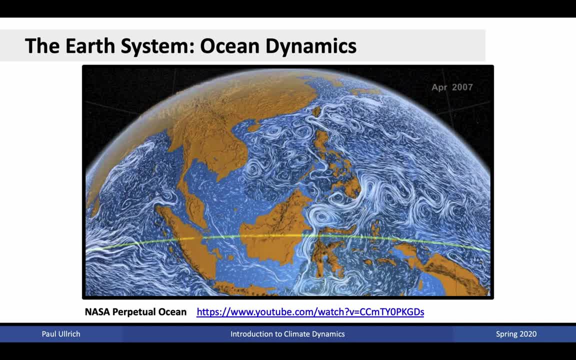 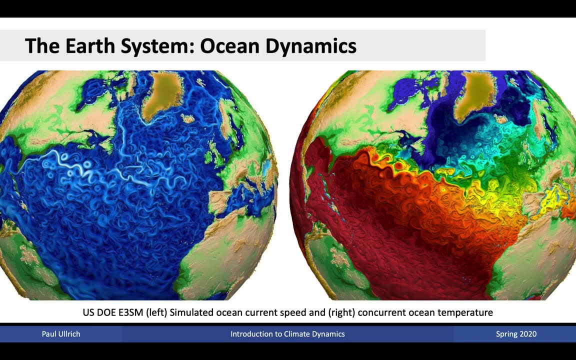 circulate oceanic waters. The ocean, much like the atmosphere, responds to the warming that comes from the sun. Later in this course we will investigate both atmospheric dynamics and oceanic dynamics. Here is another plot coming to us from the US Department of Energy E3SM model showing both simulated ocean. 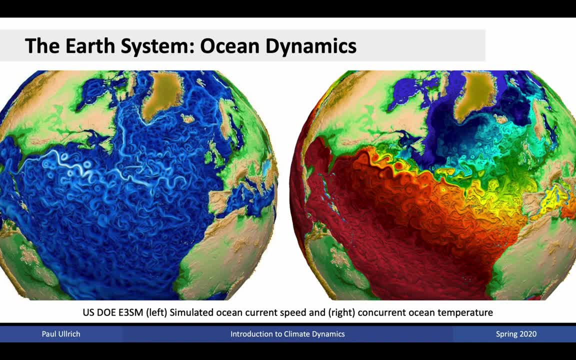 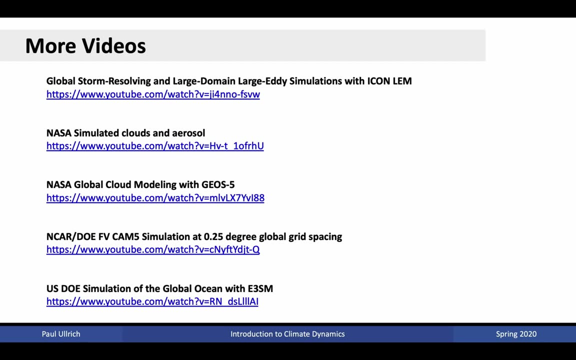 temperature, concurrent speed and concurrent ocean temperature. What you'll notice is that the small-scale eddies that exist within the ocean add a lot of fine-scale structure within the ocean. that makes it particularly interesting to study. For more videos that explore the dynamics of the atmosphere and ocean you can follow. 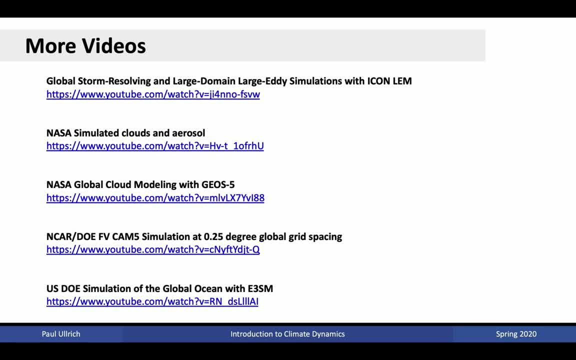 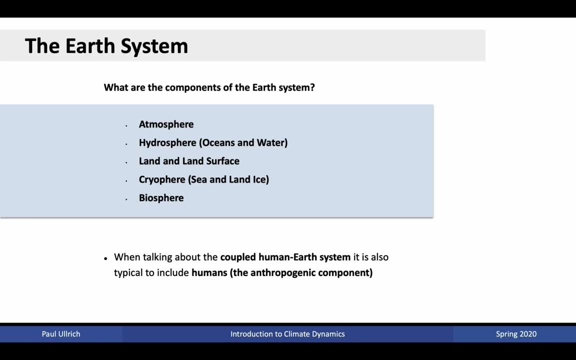 the links provided here or within the comments section of this YouTube video. Alright, let's delve into some of the academic material of this class. The first thing we want to investigate is: what are the components of the Earth system? Typically, when we talk about the Earth system, we refer to five interconnected components. 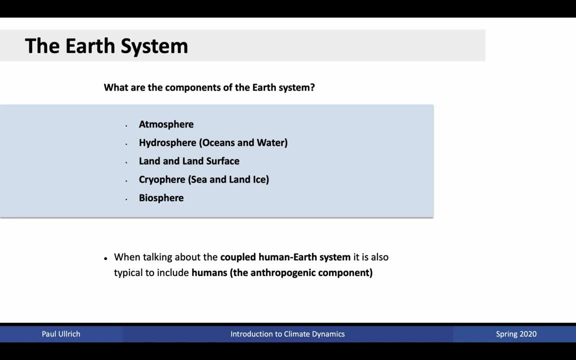 The atmosphere, describing the motion of air in the system. The hydrosphere, which includes the oceans and land water, including lakes and rivers. The land and land surface, which includes the soil layers near the surface. The cryosphere, which refers to sea and land ice. And the biosphere, which refers to. 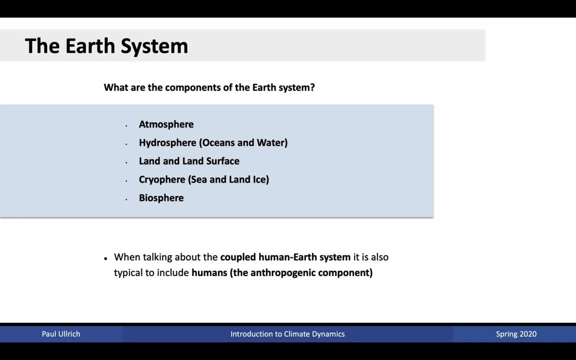 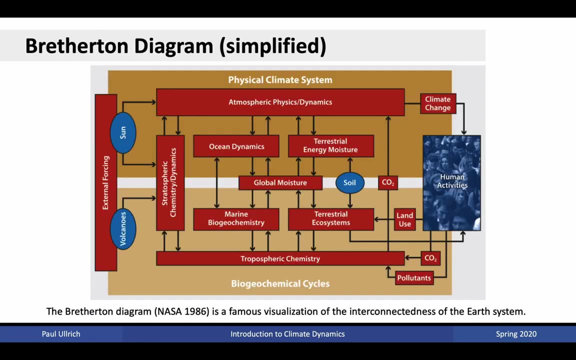 vegetation and crops, as well as fauna and flora, across the Earth's surface. When we talk about the coupled human Earth system, it's also typical to include humans, which is known as the anthropogenic component of the system. The Bretherton diagram provides a simplified overview of the interconnectedness that exists within the global Earth system. 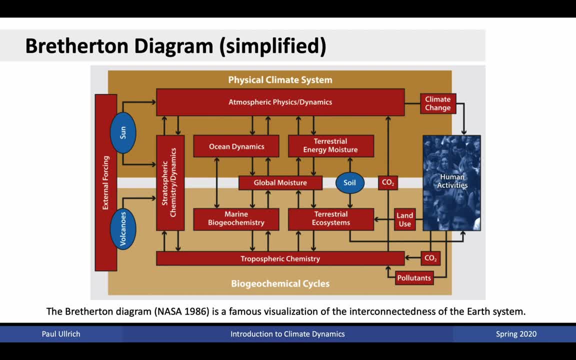 On the top of the diagram, we see the physical climate system, which is the part of the system, which is the most important component of the Earth system, which is effectively described by partial differential equations, such as the equations of atmospheric dynamics that I have talked about previously. 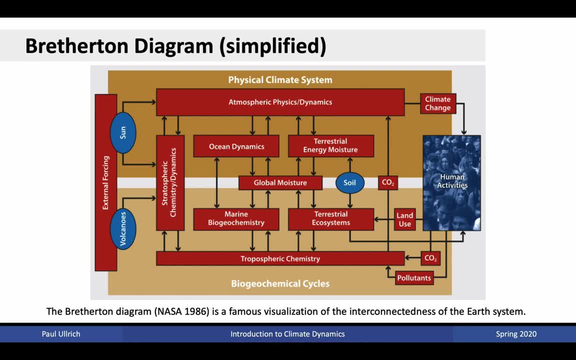 As well. the ocean is governed by similar equations, again associated with the flow of fluids. These dynamical processes that arise from these partial differential equations are then responsible for moving energy and moisture through the Earth system, but also moving chemical constituents, and hence is important for 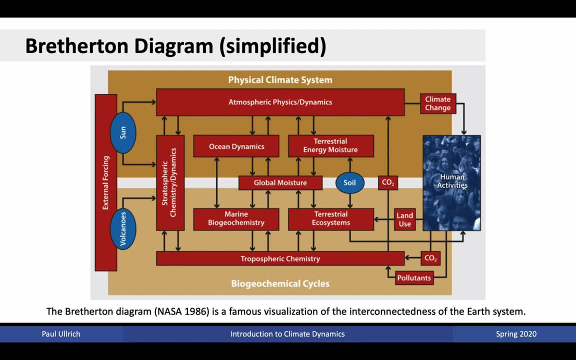 stratospheric chemistry and dynamics, as well as tropospheric chemistry and dynamics. On the left-hand side of this diagram, we see external forcing, which refers primarily to volcanoes and solar forcing. Although these are not parts of the climate system, this diagram emphasizes the fact that these are major drivers. 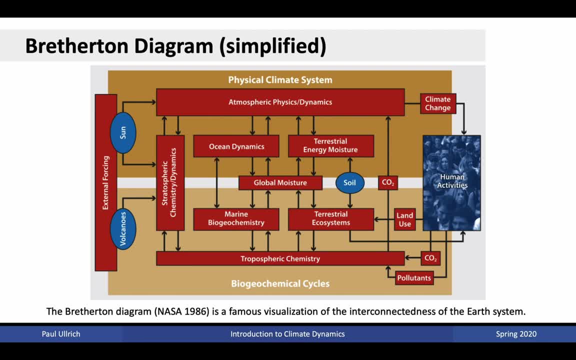 in the climate system as we experience it. The motion of moisture and energy throughout the system is then important for governing the biogeochemistry of the marine ecosystems as well as terrestrial ecosystems, and that plays a role as well in tropospheric chemistry. 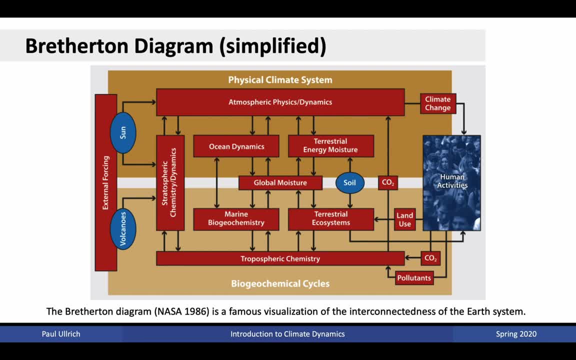 This diagram further emphasizes how human activities are interconnected with the global Earth system. We see carbon dioxide emissions and other pollutants, as well as land use, playing a role in influencing this overall system. The feedbacks associated with these activities come in the form of climate change. 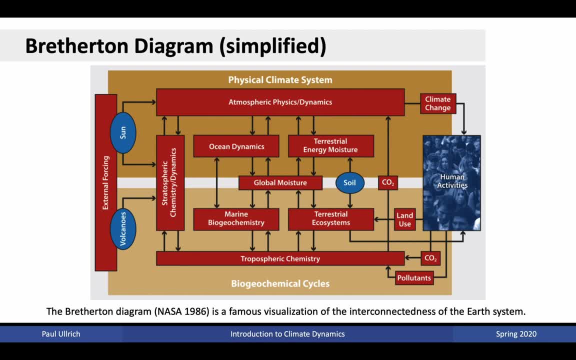 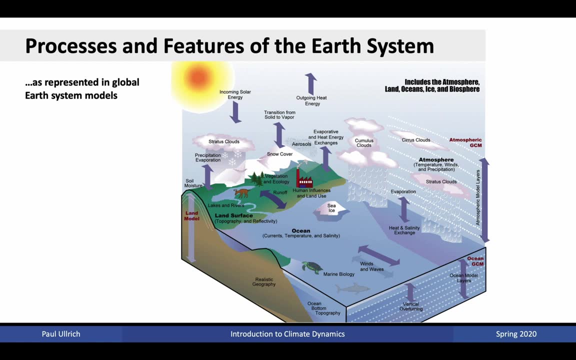 namely through our activities, we are affecting the Earth system and are consequently experiencing the Earth system attempting to equilibrate to those changes. There are many processes and features within the Earth system that emphasize its interconnectedness. Here is a depiction of some of those processes and features as they're captured in global Earth system models. 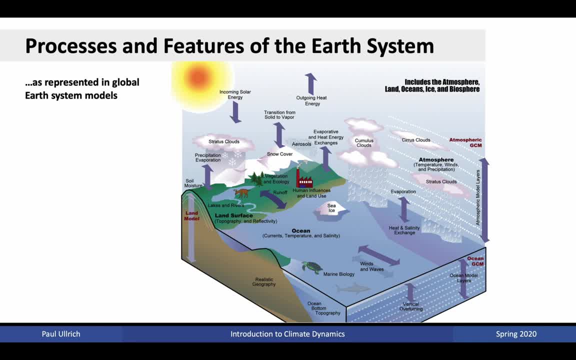 Within the atmosphere, we have temperature, wind and precipitation, as well as water vapor. With these quantities, we can learn something about clouds as well as other precipitating systems. Evaporation from the ocean is the primary driver for the addition of water vapor to the atmosphere. 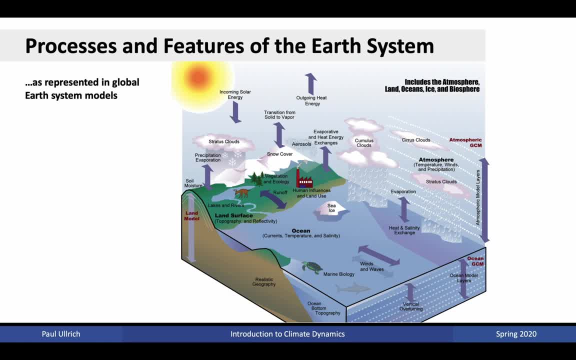 but there are other fluxes of quantities, such as heat and salinity exchange, that affect the oceanic chemistry. The exchange of energy through the system occurs through incoming solar energy, outgoing heat energy, as well as the dynamics of energy exchange across the surface. 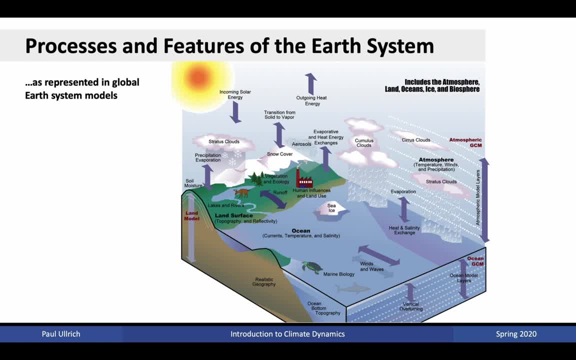 The ocean is described through currents, temperatures and salinity, which is affected by atmospheric behavior at the atmosphere-ocean interface. However, the ocean goes much deeper than that and we can see processes that occur in the depths of the ocean that are affected by even our behavior near the Earth's surface. 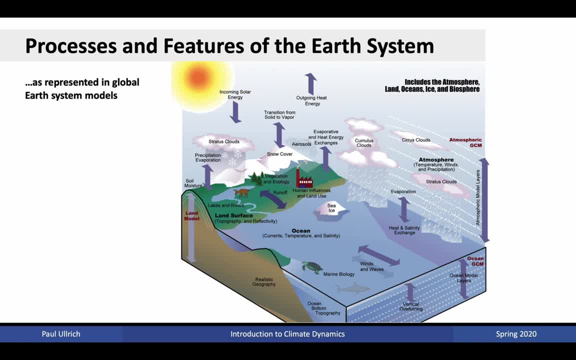 Other fine-grained features include lakes and rivers, which are responsible for runoff into the ocean, which can then affect salinity and human activities, and land use change, which are responsible for changing the reflectivity of the Earth's surface and hence modifying the overall energy exchanges that occur within this system. 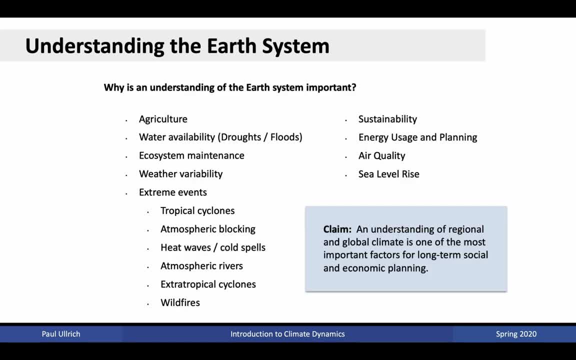 So why is an understanding of the Earth system important? I've listed here several key application areas where climate dynamics and an understanding of the Earth system is highly relevant to the discipline. When understanding cropping for agriculture, one needs to understand where one can plant crops. 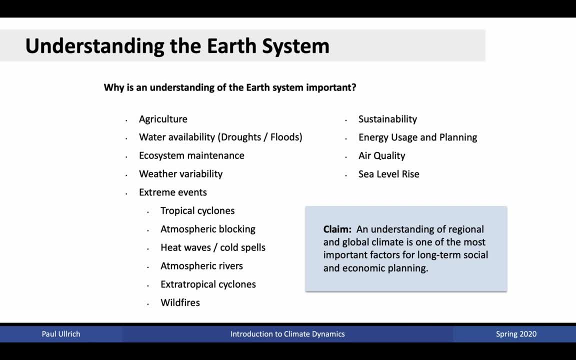 and which crops will grow in particular climate zones. When understanding water availability, we need to know how much precipitation we're going to receive, as well as evaporation of that precipitation. Also, we have to worry about extreme events, including droughts and floods associated with a lack of water or too much water. 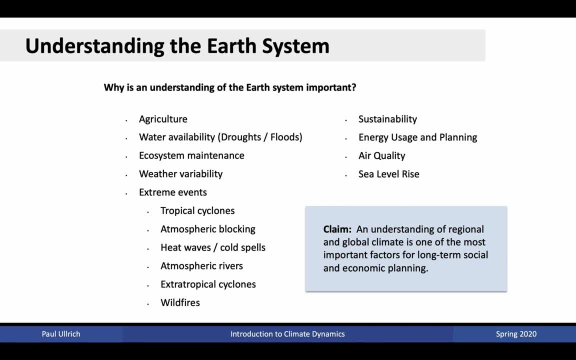 Ecosystem maintenance, which includes, for instance, the forests of montane regions, relies on soil moisture as well as precipitation, And understanding weather variability is key if we're going to understand the impacts of individual weather events. One typically does not want to live in a region where weather is extremely variable. 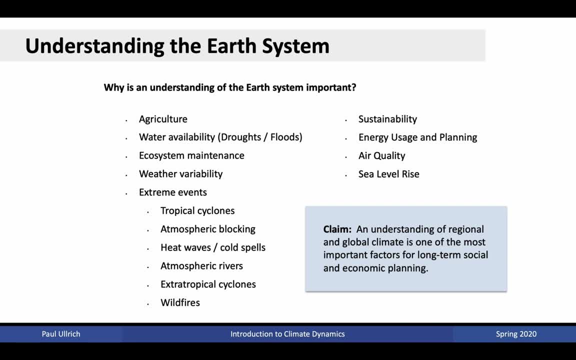 since you never know how to plan for the next day. Consequently, we're very interested in studying extreme events in the climate system, including tropical cyclones, atmospheric blocking, heat waves and cold spells, atmospheric rivers, extra-tropical cyclones, which are responsible, for instance. 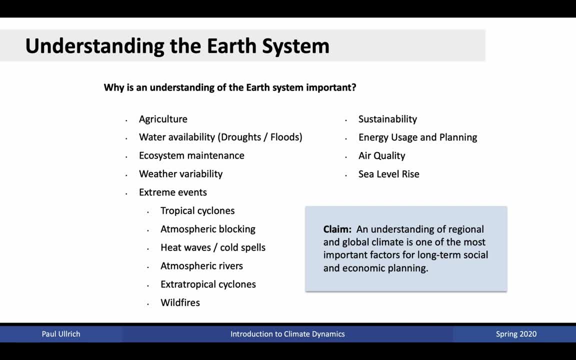 for wintertime storms as well as wildfires. We're also interested in sustainability, namely, how can we live sustainably within the Earth system and ensure that through our activities we're not irreversibly modifying that system? We want to understand energy usage and planning. 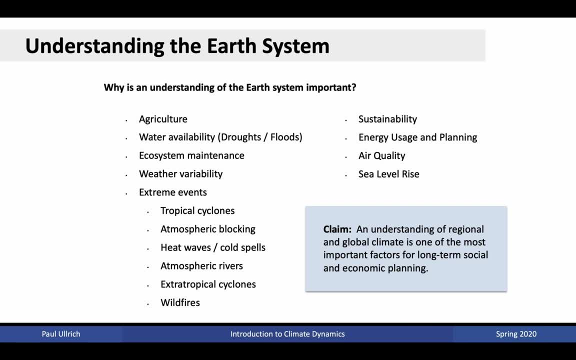 for instance, where to locate solar panels, where to locate solar power plants, where to locate hydroelectric power plants, such that they're resilient to future change. We want to understand air quality, because of impacts on human health. We want to understand sea level rise because of danger to our coastal communities. 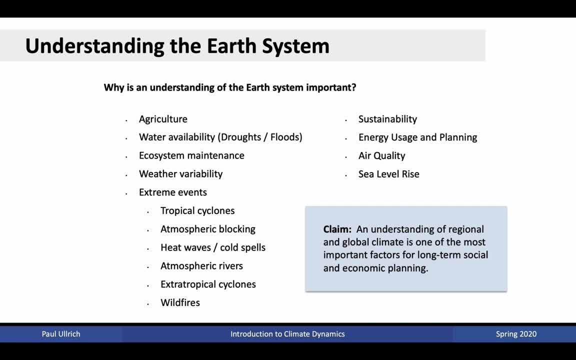 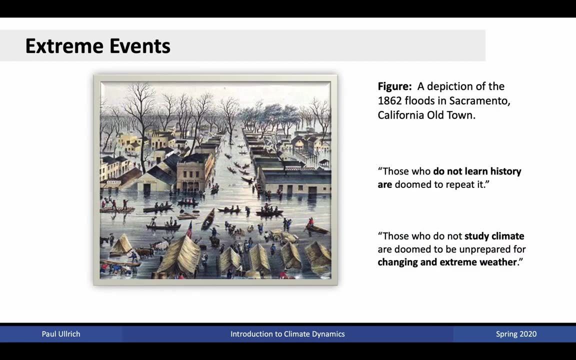 All of these application areas are intimately connected with climate dynamics, And so an understanding of regional and global climate is arguably one of the most important factors in social and economic planning and needs to be incorporated in any sort of long-term plan. Here is a depiction of the 1862 floods that occurred in Sacramento, California, Old Town. 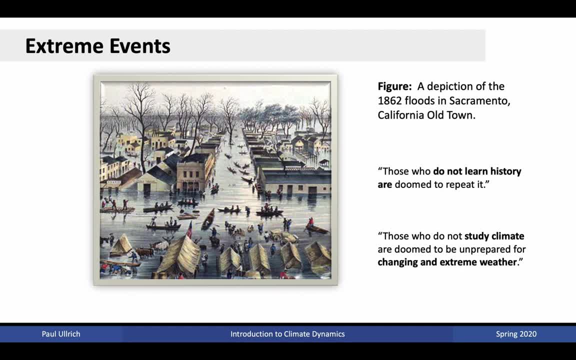 This was a very rare event and one that has not occurred since, but one where the extent of the damage was sufficiently severe that it was felt for many years after that and became a key event for future planning. Similar events such as this may be coming in our lifetime. 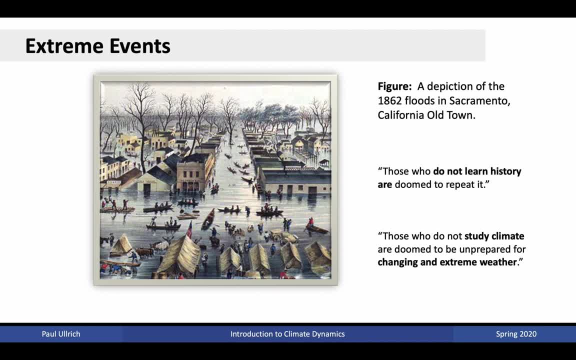 However, without understanding climate dynamics and without understanding the climate system, we cannot predict the likelihood of one such event. Consequently, there is a familiar adage that says: those who do not learn history are doomed to repeat it. I would argue that there is an analogous statement. 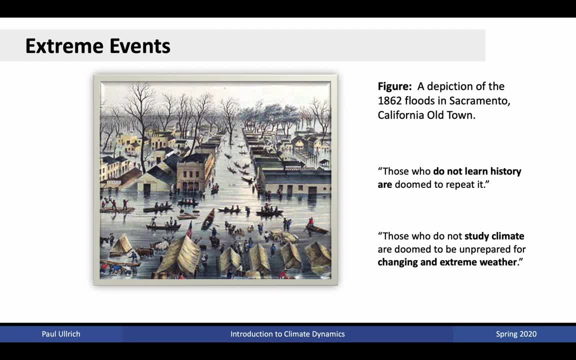 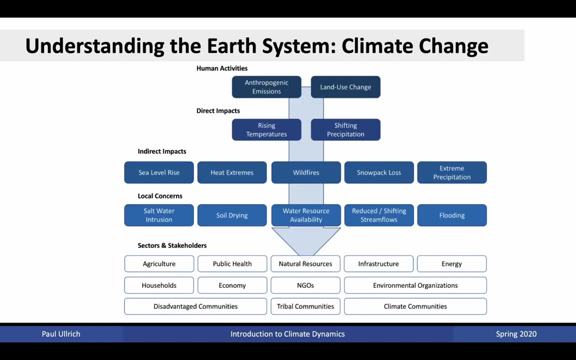 to be made about climate dynamics. Namely, those that do not study climate are doomed to be unprepared for changing and extreme weather. We need to know when the next extreme weather event will come so that we can be prepared accordingly, As we understand the Earth system. 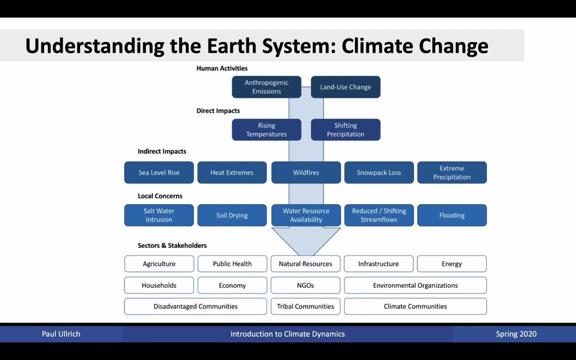 we also need to investigate how human activity is impacting the Earth system. Human activities are typically through anthropogenic emissions and land-use change, which affect tropospheric chemistry as well as affecting reflectivity of the underlying Earth's surface. These two then result in changes to energy balances within the system. 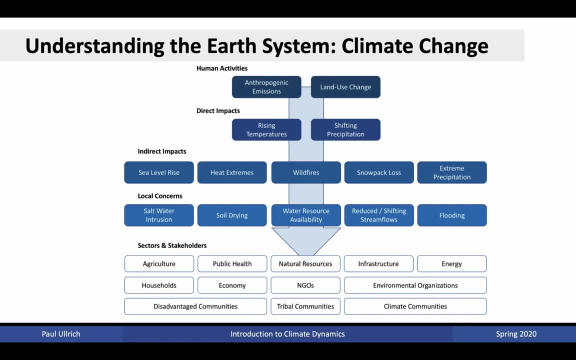 In this class, we're going to understand how energy moves throughout the system and, consequently, how that system will respond to both anthropogenic emissions and land-use change. The direct impacts of climate change are rising temperatures and shifting precipitation patterns, which then have indirect impacts to sea level rise. 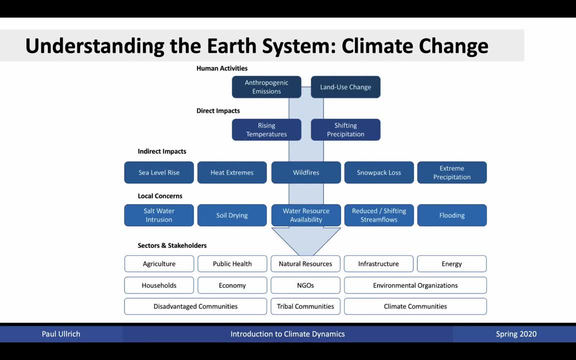 heat extremes, wildfires, snow plaque loss and extreme precipitation At the local level. an understanding of climate change is then important for understanding saltwater intrusion, which can impact water availability as well as soil drying. other water resource availability reduced, shifting streamflows as well as flooding. 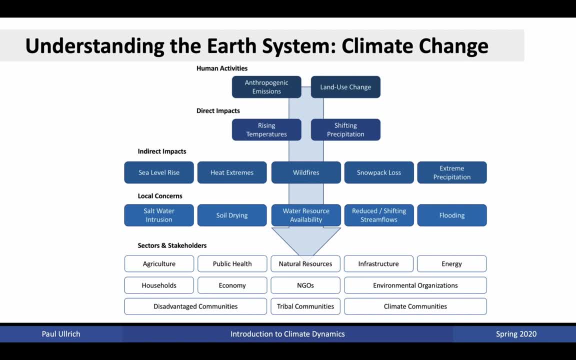 All of these play then into various sectors and stakeholders which are then interested in behavior of the climate system, including agriculture, public health, natural resources, infrastructure, energy, as well as many of the other sectors and stakeholders listed here. Many of these communities are investigating. 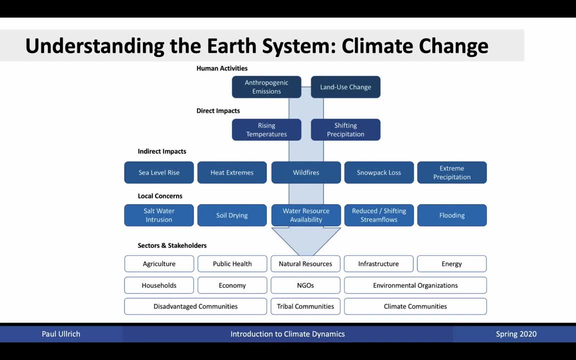 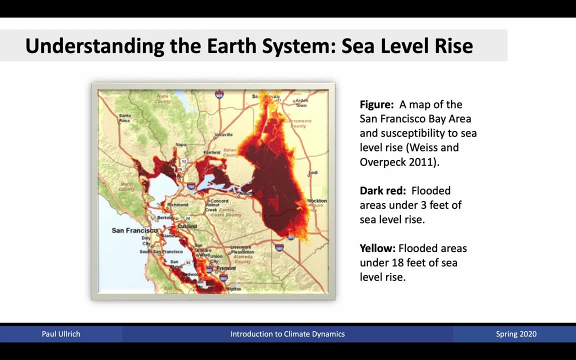 how climate changes will be affecting them over the next 100 years and are planning accordingly. Sea level rise in California is, in particular, a major worry. With only three feet of sea level rise, most people do not realize that much of the area around the San Francisco Bay will be flooded. 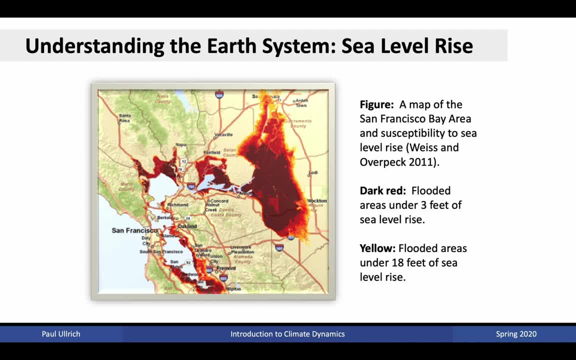 But not only that, but through much of the Central Valley there are large sections of land that are below three feet above sea level. These areas would be flooded very readily, And it turns out even that under about nine feet of sea level rise. 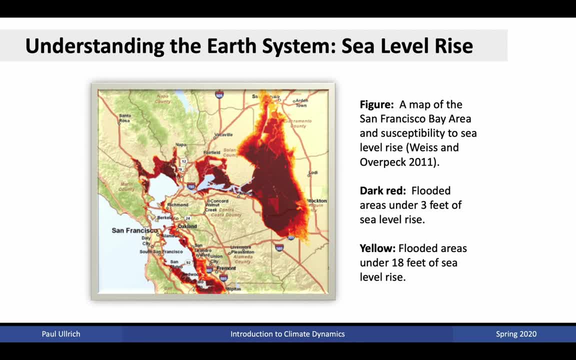 what we will see is the San Francisco Bay extending as far north as Sacramento. By understanding and projecting how high sea level will rise in response to changing temperatures, we will then be able to plan accordingly for sea level rise and not place, for instance. 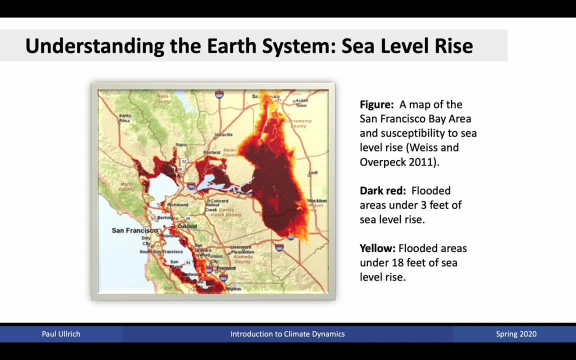 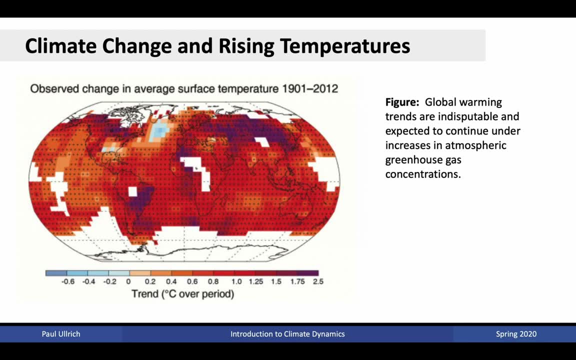 our coastal infrastructure in dangerous places. Climate change and rising temperatures is important worldwide and this is one of the biggest challenges of our time. Global warming trends to date have been indisputable, particularly those since the 1970s. In particular, we're seeing very pronounced warming. 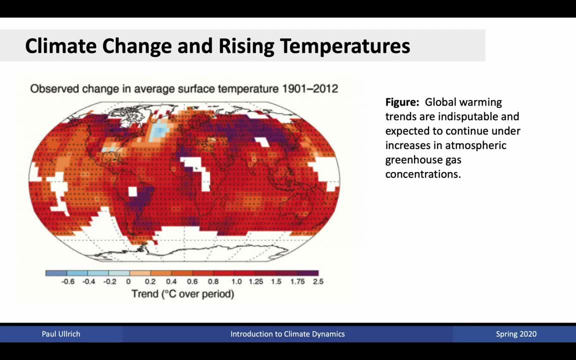 occurring at the very northernmost latitudes. What this means is that there is a change in the distribution of energy and moisture in the Earth's system, and this will in turn affect again heat waves and precipitation patterns. Throughout this course, you will learn about the different processes. 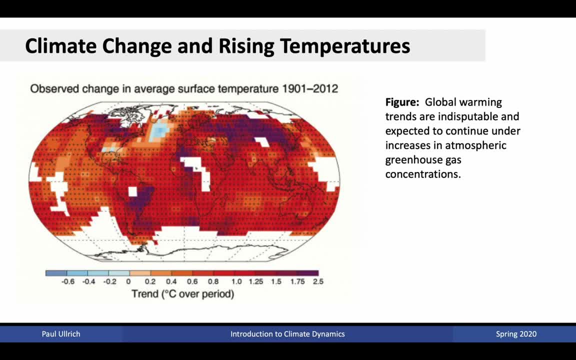 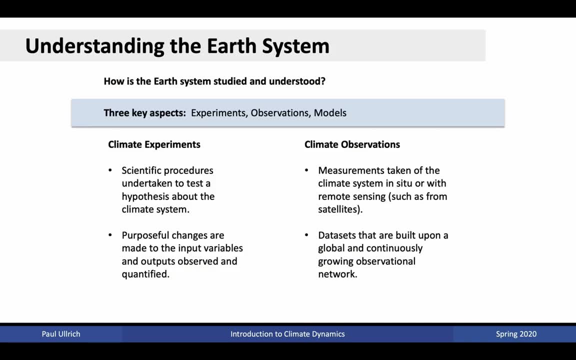 by which energy and moisture are exchanged through the Earth's system and, consequently, how we anticipate those processes to respond to climate change. So how do we go about understanding the Earth's system? There is a way to break down our understanding into three key aspects. 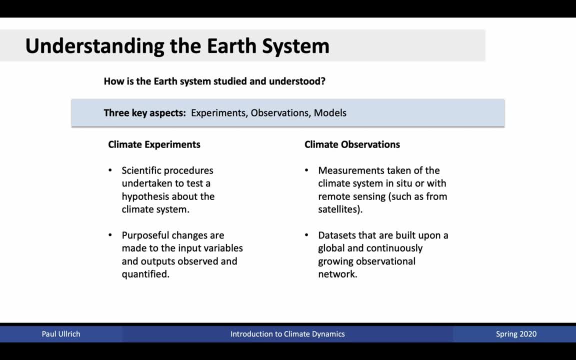 Experiments, observations and models. Climate experiments refer to scientific procedures that are undertaken to test a hypothesis about the climate system, as well as purposeful changes that are made to input, variables and outputs observed and quantified. Observations, on the other hand, are more passive. 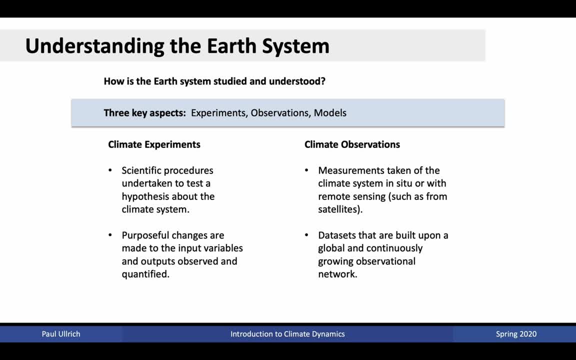 but they exist in basically a vast worldwide network. These measurements are either taken in situ, that is, in place, or with remote sensing, such as with satellites. Since 1979, we've had access to a vast amount of data from a global satellite network. 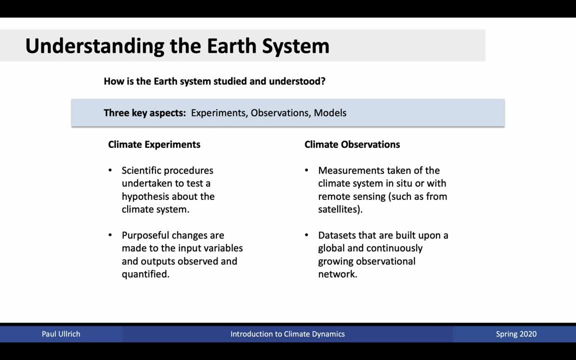 that has provided constant observations looking down on the Earth's surface. This vast trove of data has provided us with indispensable insight into how the climate system behaves. Consequently, we have massive data sets built upon a global and continuously growing observational network of the Earth's system. 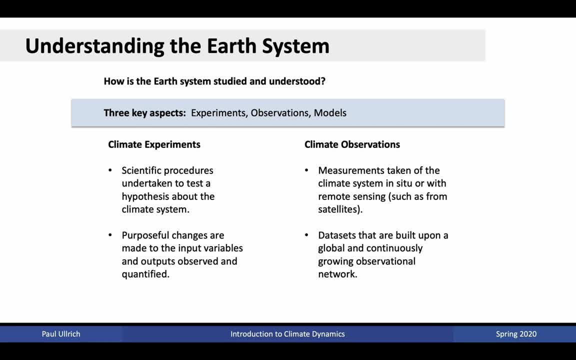 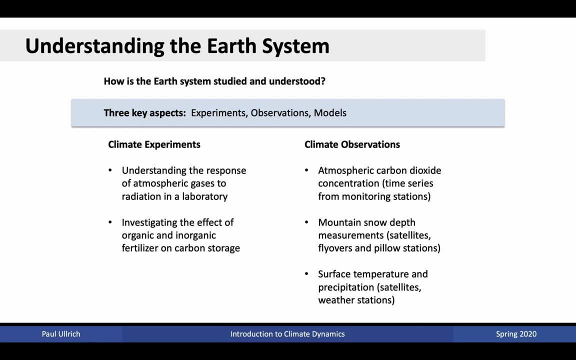 And this continues to today- to inform our understanding of the climate system. Examples of climate experiments include understanding the response of atmospheric gases to radiation in a laboratory. What we'll investigate in this class is how the chemical composition of the atmosphere plays a role in affecting energy redistribution. 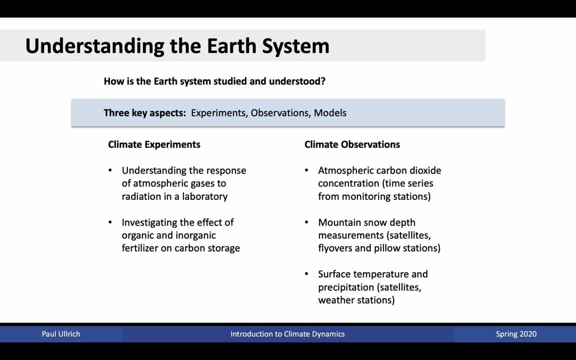 And much of this can be studied in a laboratory by simply shining light through gaseous chambers. We also include climate experiments, such as investigating the effect of organic and inorganic fertilizer on carbon storage and investigating how the carbon cycle is important in modulating the amount of carbon. 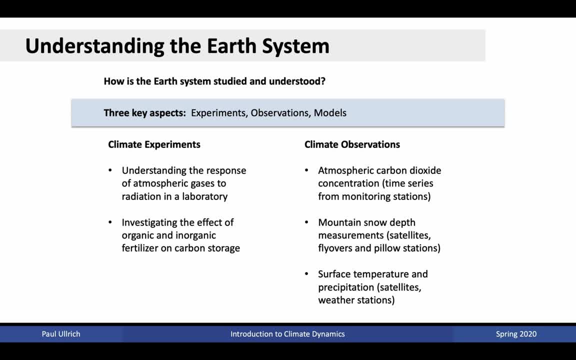 that is present within the global climate system. As I mentioned previously, there is a vast network of climate observations investigating everything from atmospheric carbon dioxide concentrations that have existed since the 1950s, as well as time series from all over the world. We also have measurements of mountain snow depth. 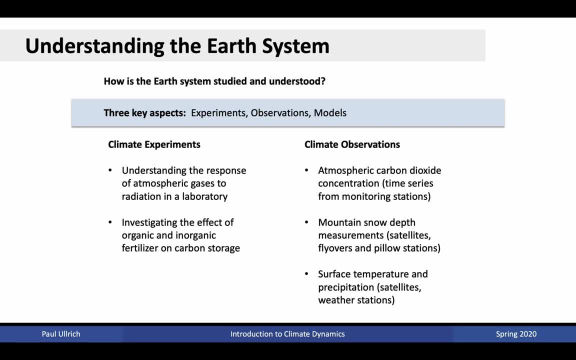 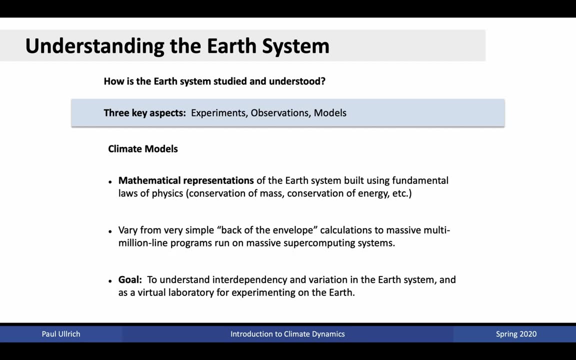 including satellites, flyovers and pillow stations, as well as meteorological stations that have existed for over 100 years measuring things like surface temperature, pressure and precipitation, as well as satellite observations that continuously provide us with up-to-date information on our climate system. 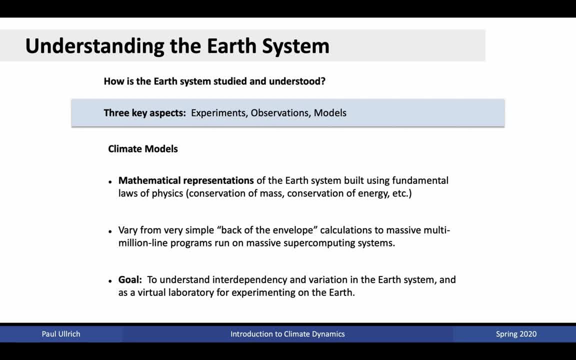 All of this information then propagates into climate models. You may have heard of climate models in the context of the IPCC assessment reports, for instance, which amalgamate years and years of study into the climate system. Climate models, though, are computational systems. 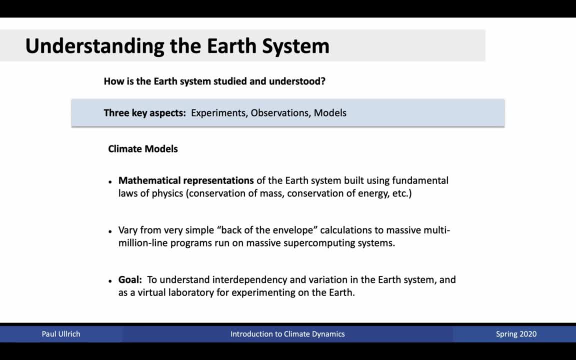 or mathematical representations of the Earth's system that are built on fundamental laws of physics, as well as our understanding of the global climate system. Using experiments and observations, we can constrain climate models and build the best possible representation of the Earth's system that we can. 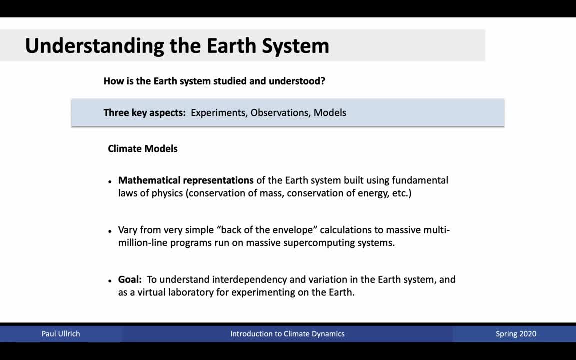 And then execute this model on large-scale supercomputing systems, which then give us insights into the behavior of the Earth's system. However, there are also very simple back-of-the-envelope type climate models that we can use to build a deeper understanding of energy and moisture exchanges in the system. 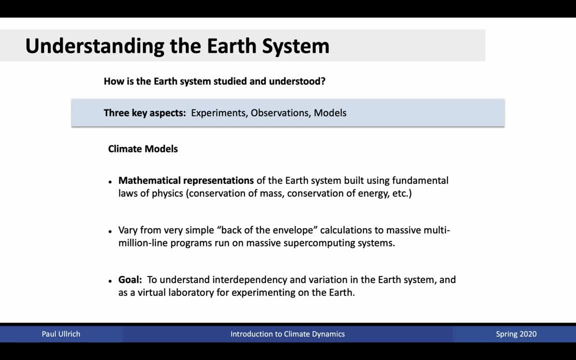 And we'll be investigating in this class some of those simpler climate models. The goal of climate models overall is to understand the interdependency and variation in the Earth's system, to provide a virtual laboratory for experimenting on the Earth, as well as provide us with a method. 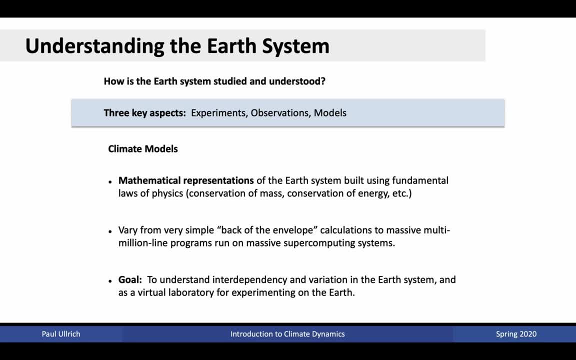 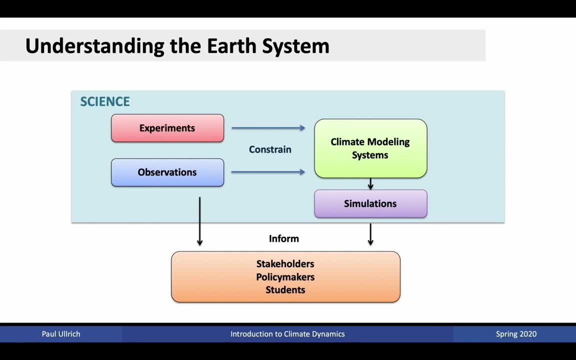 of evaluating how much we actually know about the Earth's system. So, if one was to depict this as a flowchart, experiments and observations are taken in order to build data on the Earth's system that then constrain our climate modeling systems that in turn provide simulations. 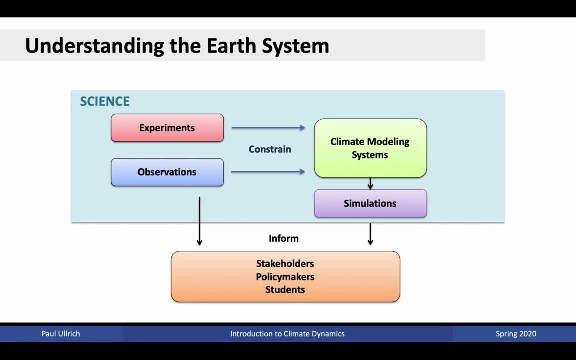 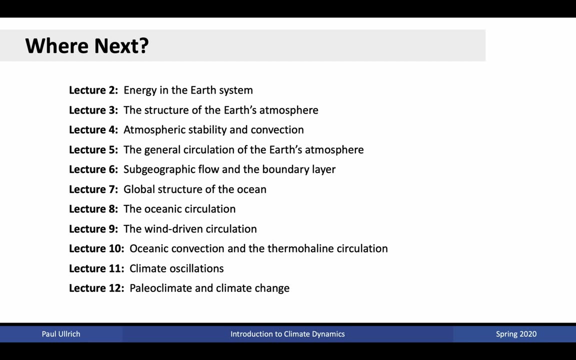 and then observations and simulations. together allow us to inform stakeholders, policy makers and students, and consequently allow us to plan for an uncertain future and a changing climate. So where are we next in this class? In Lecture 2,, we'll investigate energy in the Earth's system. 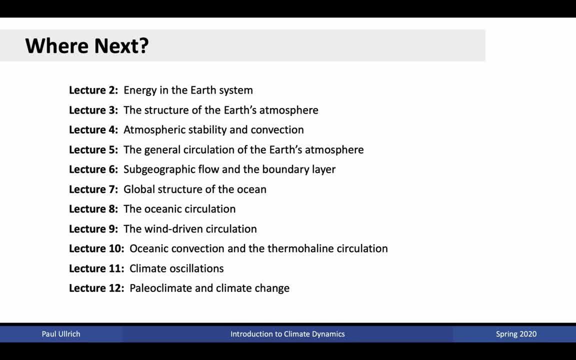 In Lecture 3, we'll talk about the structure of the Earth's atmosphere. Then we'll talk about atmospheric stability and convection, investigating the atmosphere's moist processes. In Lecture 5, we're going to talk about the general circulation of the Earth's atmosphere. 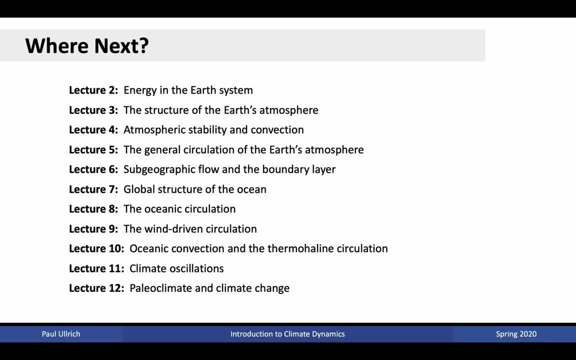 In Lecture 6, we're going to talk about the sub-geostrophic flow and the boundary layer, again extending on some of the concepts from atmospheric dynamics, and then investigate how the atmosphere-ocean coupling works, specifically investigating how the interconnectedness 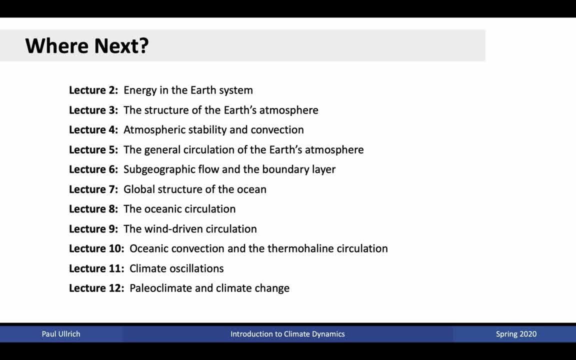 between the atmosphere and ocean gives rise to the global structure of the ocean. We're then going to investigate the oceanic circulation, as well as delve deeper into how the atmosphere and ocean are connected with one another through the wind-driven circulation. We're then going to talk about oceanic convection. 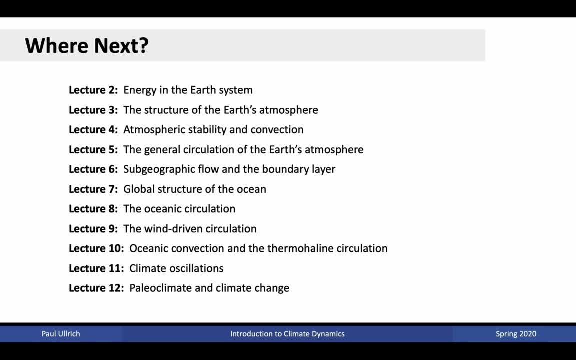 and the thermohaline circulation. We're going to talk about climate oscillations, and then we're going to finish off discussing paleoclimate and climate change. As time allows, we may discuss additional topics, So that's all for today. 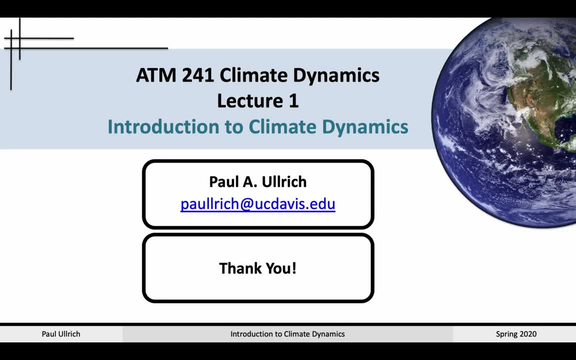 Thank you very much for listening and I look forward to talking to you guys next time.